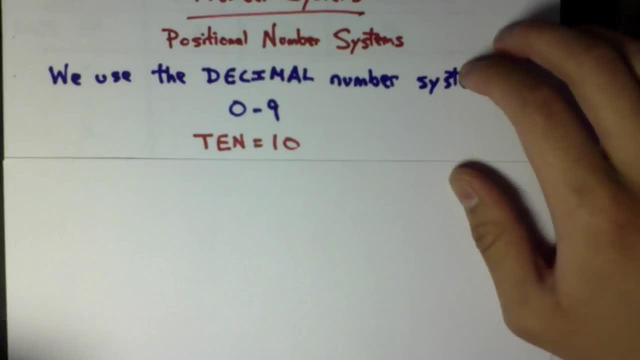 Now, when we get to number 10, we don't actually have a single digit that represents 10, so instead we choose to represent it as a 1, followed by a 0. Now why do we do that? All will be explained when we think about what a positional number. 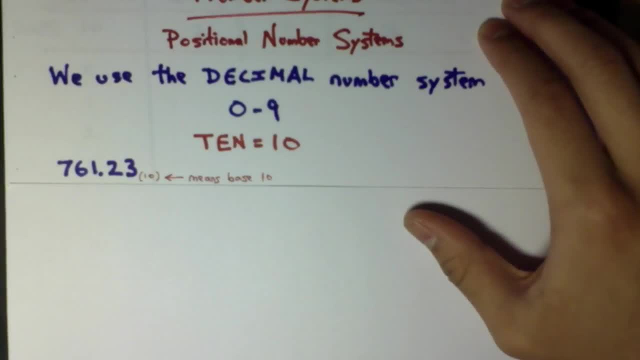 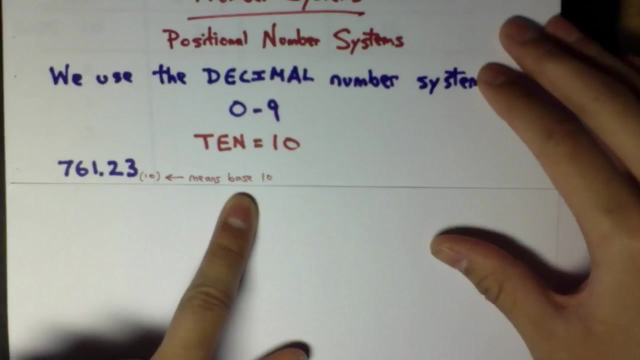 system actually is. So I want you to look at this example: 761.23.. The subscript here with a 10, denotes what base we're in. Base 10 is what we use on a day to day basis, So this number here can. 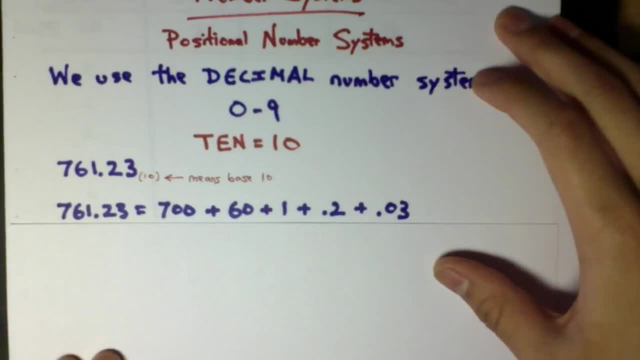 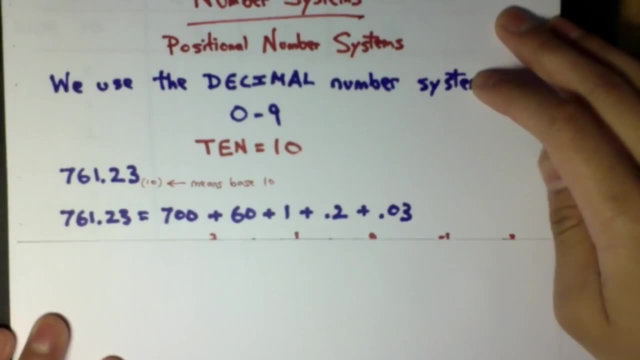 be represented as 700 plus 1.. Plus 60 plus 1 plus 0.2 plus 0.03.. Now, why do we want to do this? Well, if we factor out the 10 in each number, what we obtain is 7 times 10 squared plus 6 times 10 to the. 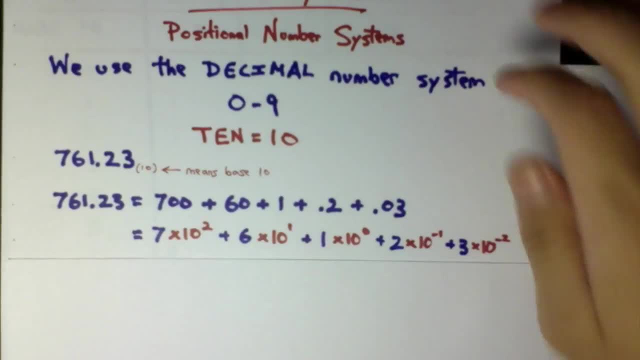 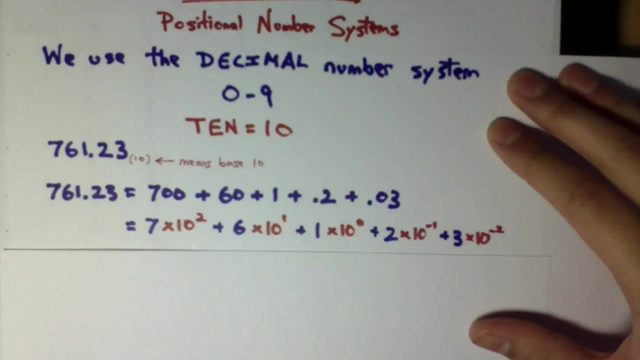 power of 1, and so on. What this represents here is that it illustrates that each digit depends on its position relative to the decimal point, which is very important in how we're going to be applying these to different bases. So Now that we've already established what base 10 is, that we have 10 different numbers in. 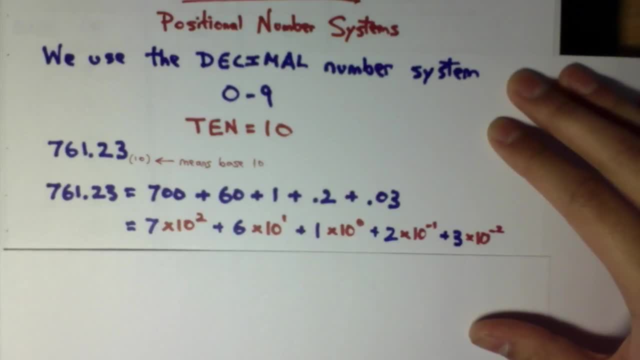 our system digits 0 through 9, it's time to take a look at different number bases. So, to start, let's take a look at base 2.. Base 2 is known as binary and, following the same concept, instead of having 10 different numbers in base 10, base 2 has only two different. 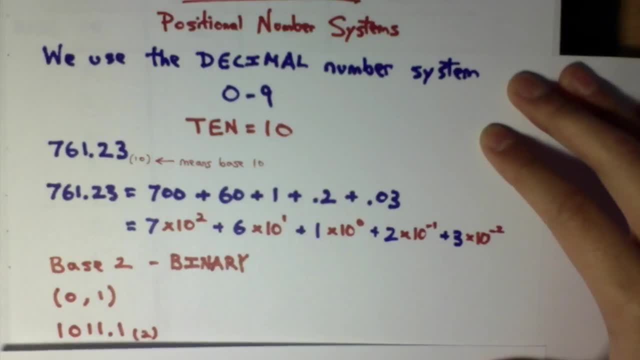 numbers 0 and 1.. Base 2 is referred to as a binary system, and the reason why it is so important is because it is the basic unit of information in computing and electrical communications. In electronics, there are simply two states: on or off. 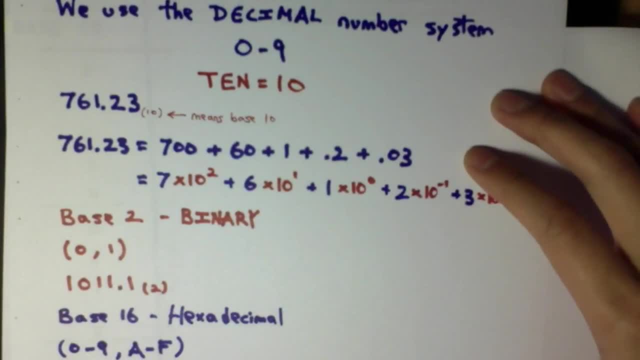 Another base that is very important is base 16, known as hexadecimal. In hexadecimal, we have more digits than we're used to. So to represent these, we're going to use the hexadecimal. So to represent these, we're going to use the hexadecimal In hexadecimal, we have 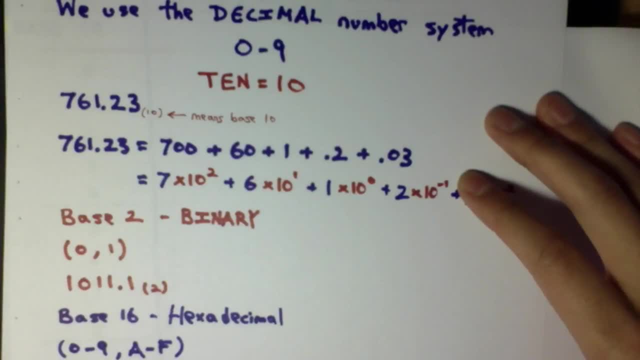 more digits than we're used to. So to represent these, we're going to use the hexadecimal. So to represent these, we're going to use the hexadecimal. So to represent these, we're going to use the hexadecimal. But since we need 16 of them, we use letters a through f to represent the other missing. 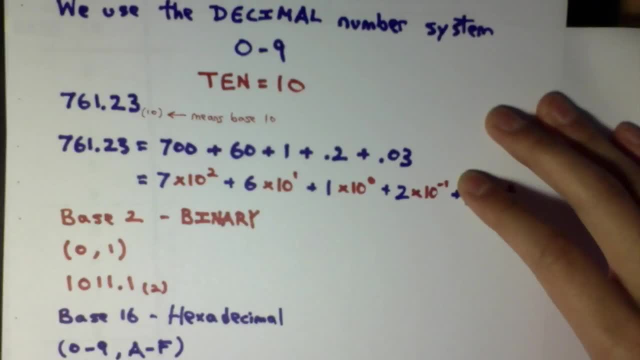 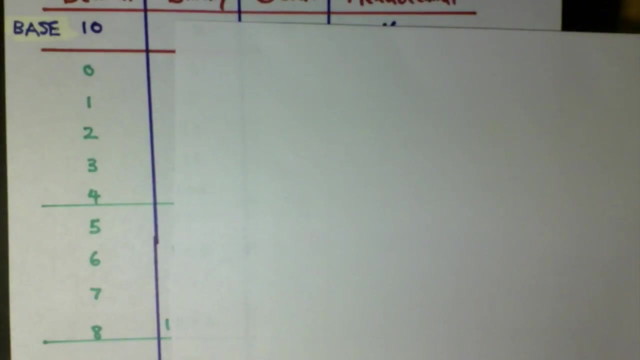 numbers. So in this case, a represents 10,, b represents 11, and so on to f equals 15.. So an example of what these numbers can look like is close Distribche contention. So now that number systems are introduced, a clearer way of understanding how different 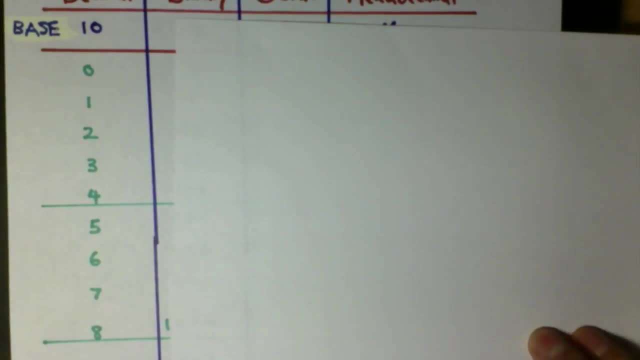 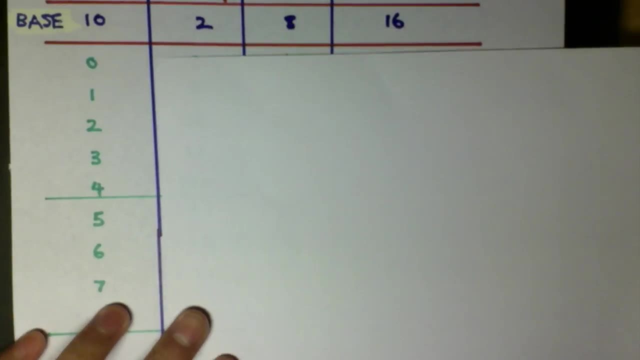 bases will work is to count in them. So what I have here is a table showing this column, showing decimal numbers, and I'm going to be looking at what these numbers are represented, as in different bases. So, for example, if we're looking at a binary system, we have only digits 0 through 1, right. 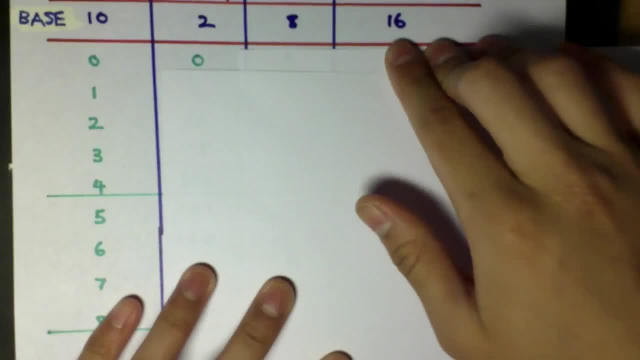 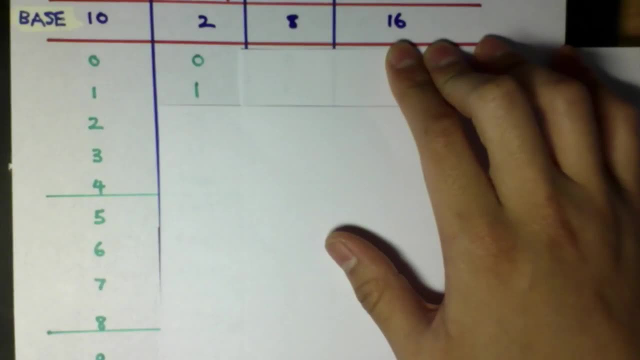 So to represent the first number, we have 0.. The next number would be 1.. But the problem is in binary we don't have the digit 2.. So to represent the next number, we have to move the 1 to the next position and we have 10.. So it seems like this number is 10, but 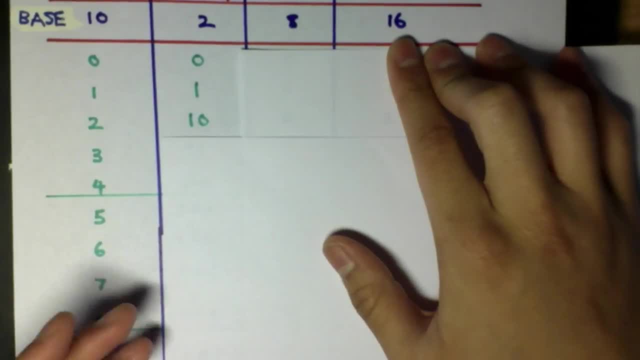 in binary it actually represents 2.. So the next number following would be 11.. And again, we don't have any other digits to use, So we have to move the 1 over to the next position and add zeros. So if we follow these rules, we have 101 is. 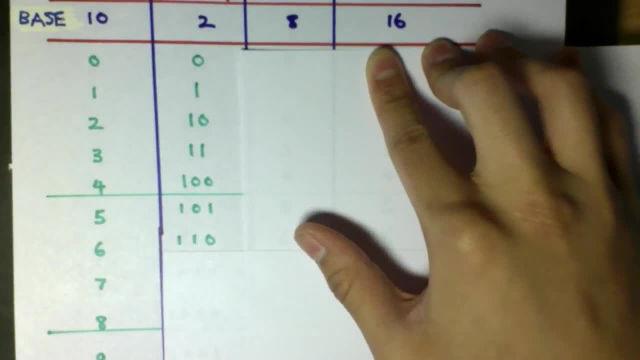 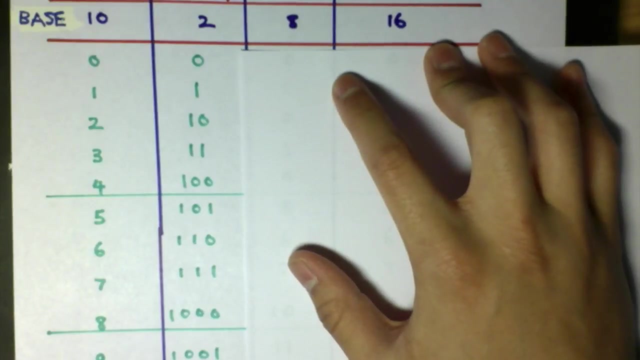 5.. 110 is 6. And 111 is 7.. Again, we have no more digits to use. So then we go to 100 and 1001.. Excuse me, 1000.. So later on we will be learning how to actually go from binary numbers to decimal numbers. 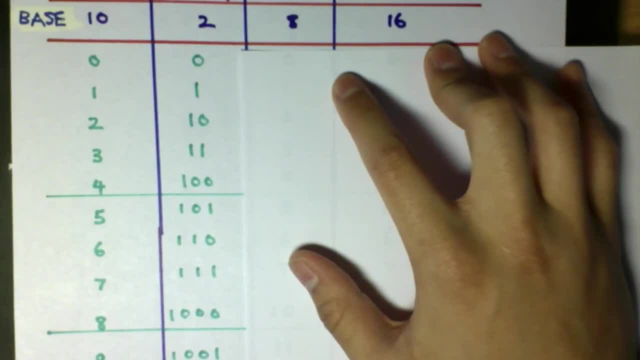 and different bases. we can swap in between too, But for now just understand the concept of going from just counting, Just counting in different bases. So now let's take a look at the octal system. If you take a look at the octal system, we 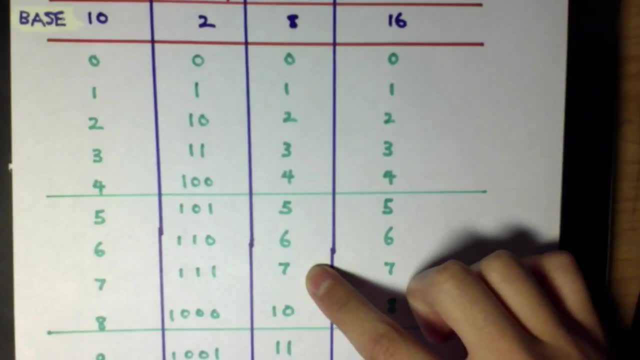 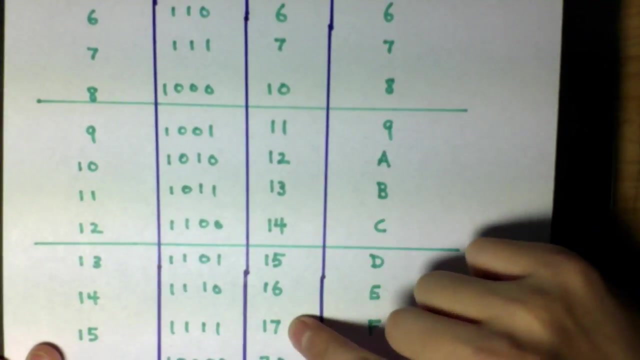 have 0 through 7 as our normal digits, But since there's no 8, that is represented in octal, since we only have digits 0 to 7, the next number following will be 10, which represents 8.. And if you go down the list, we can see that it goes to 17.. And since there's no more, 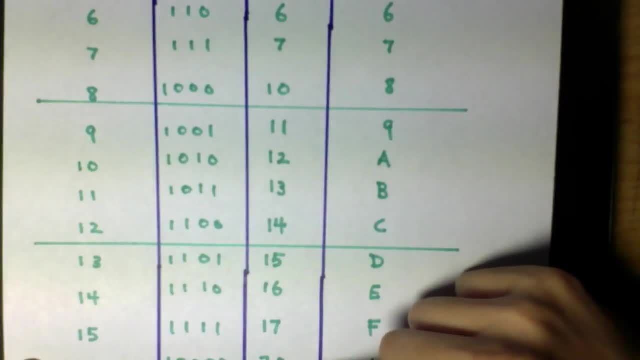 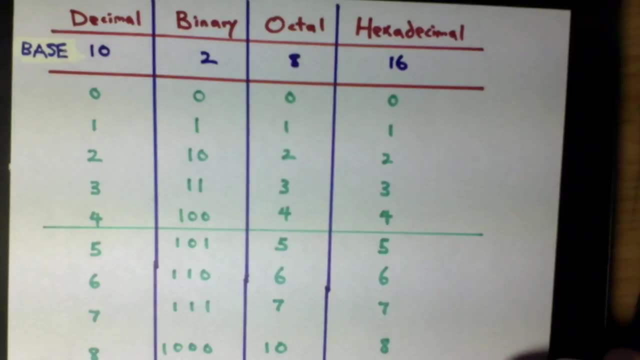 digits that follow. we have 2,, 0, and 16.. Now take a look at what's happening in the hexadecimal column For digits 0 through 9, we have the same numbers, but this time for digits 10 through 15,. 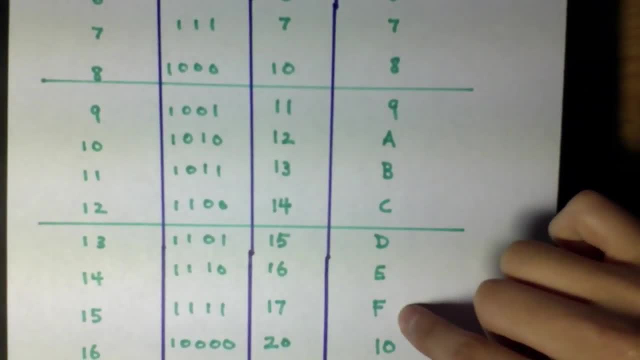 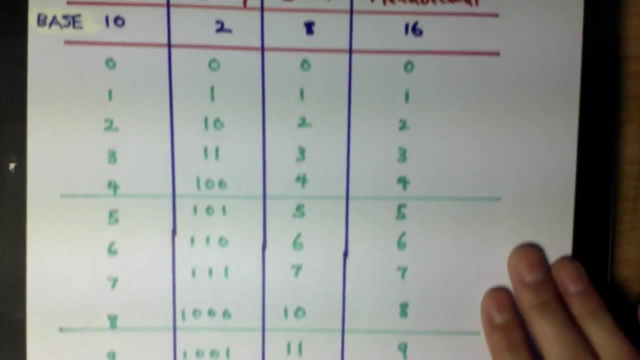 we have letters A through F that represent each of those numbers individually. Now that at 15, since there are no more digits that follow F, we represent 16, or the next number as 1, 0. So hopefully this made it clear on what number systems are and how counting on them actually. 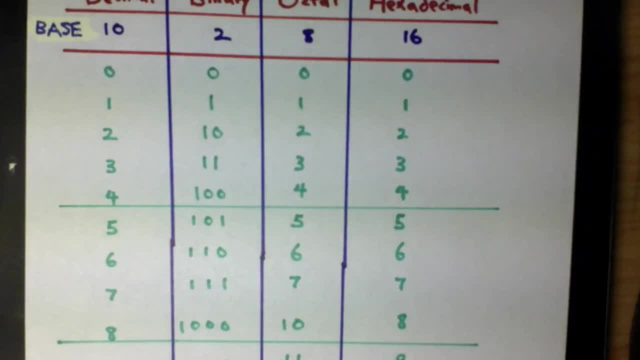 work. In following videos we'll be learning about how to go from one base to another and how there are different techniques and methods for those. 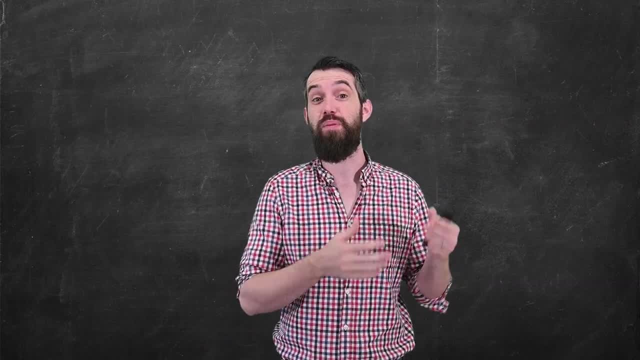 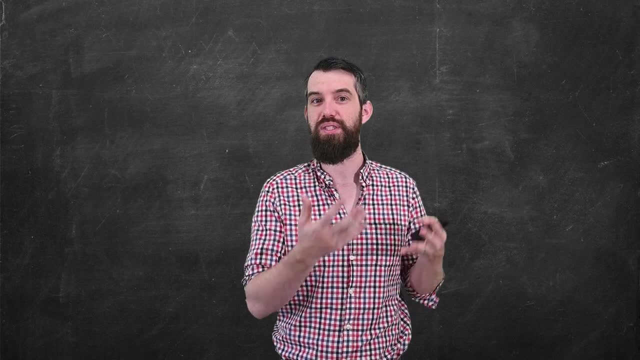 How should we define differentiability for a multi-variable function? In this video we're going to look back at single variable calculus and try to figure out what problems differentiability was trying to solve, and try to solve those same problems in the higher dimensional analog. 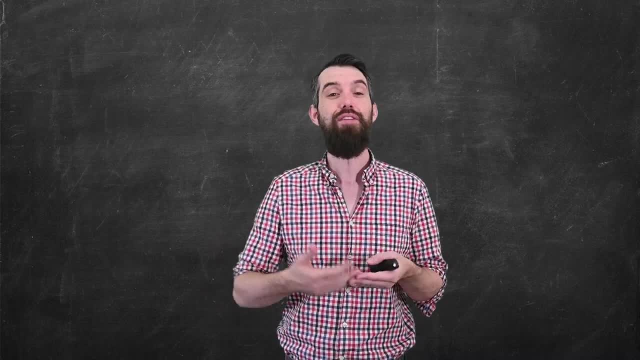 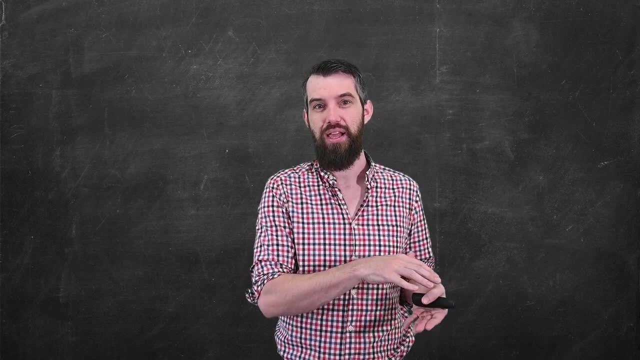 And I'll note that in the previous video, we saw that, even if partial derivatives existed, this wasn't perhaps enough to get to a full notion of differentiability, And so we really need to do something more. That's what the point of this video is, So let's begin our journey into 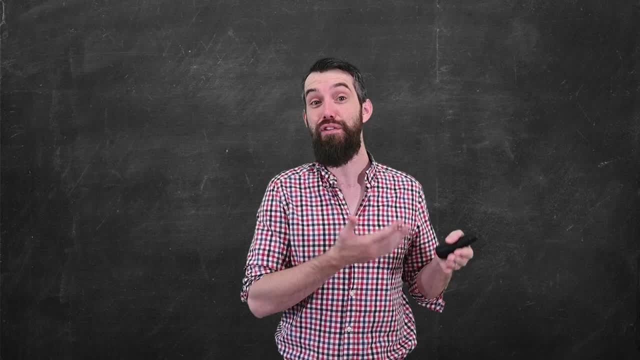 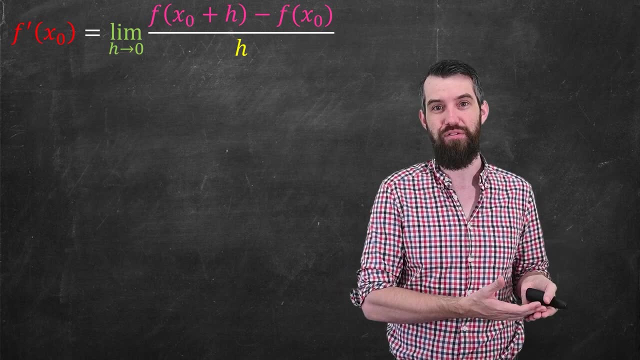 differentiability of multi-variable functions by looking at single variable functions first to build up some intuition. So let's just remind ourselves about the definition of the derivative, A few different components. We're going to say the derivative of the function. at some point x naught. 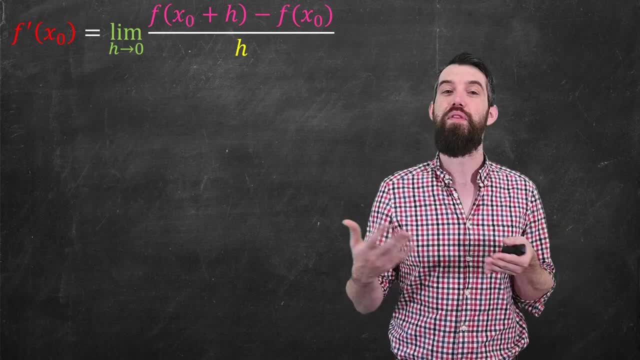 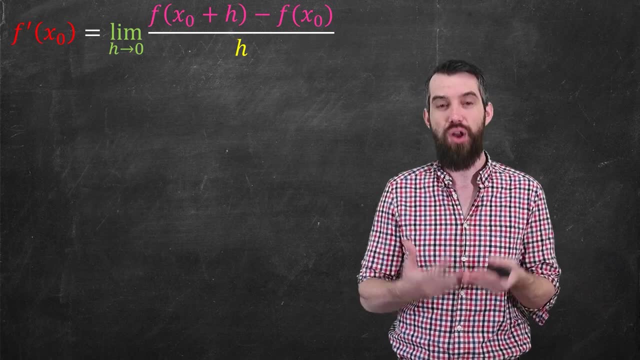 was the limit, as h goes to zero, What I call the difference quotient. The numerator has this difference- f of x naught plus h minus f of x naught, And the denominator has the value of h. Now, this formula is all fine, but what I really want to illustrate,